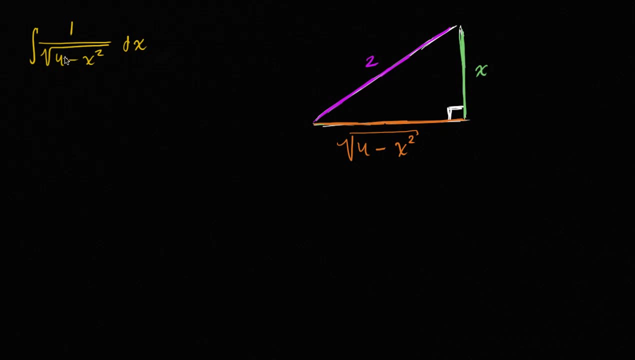 Well, that's interesting, That is this expression, that insight and intuition that we may have had when we saw this right over here. but still, how does that help us? Well, this is where the trigonometry comes in, because if we define, if this angle right over here, 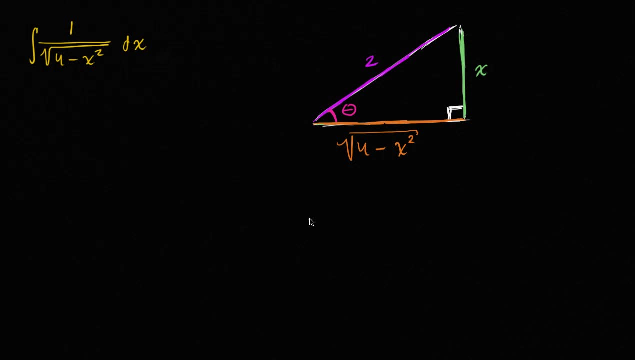 we say this is theta, then what is sine and cosine of theta going to be in terms of these sides? Well, let's see the sine of theta. sine of theta is equal to the opposite over the hypotenuse is equal to x over two. 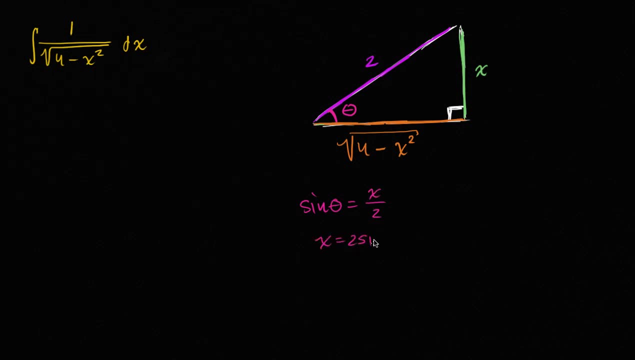 or if you want to solve for x, we get. x is equal to two sine theta. Well, that's interesting. What about the cosine of theta? Cosine of theta is equal to the adjacent side square root of four minus x squared over the hypotenuse. 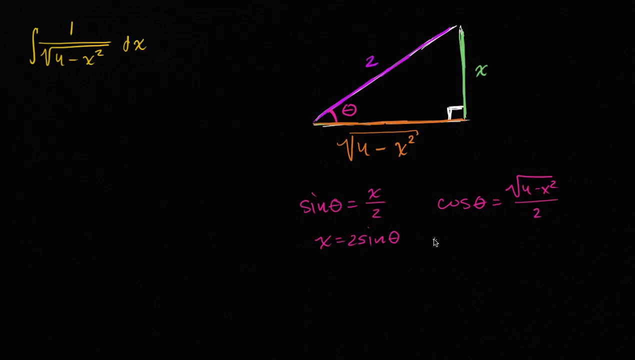 or, if you want to solve for this side it's going to be. we could say that the square root of four minus x, squared, is going to be equal to the hypotenuse times, the cosine of theta. So that's interesting if x is equal. 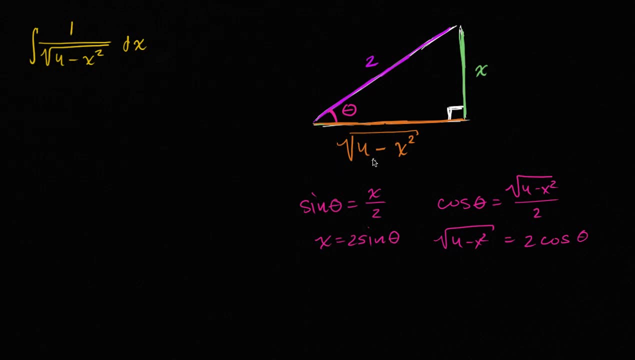 to two sine theta, then this other side, then this entire expression simplifies to two cosine theta. And that seems pretty interesting now. So let's make the substitution. Let's say that x is equal to two sine theta, and if x is equal to two sine theta, 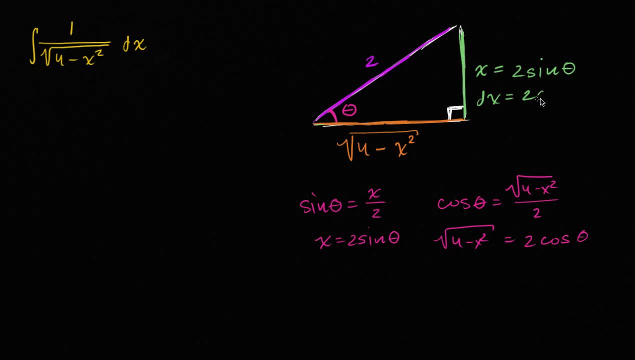 then dx is going to be equal to two cosine theta, d theta. And then if x is equal to two sine theta, then what is this thing right over here? Well, we just figured out. this thing is two cosine theta. This thing is equal to two. 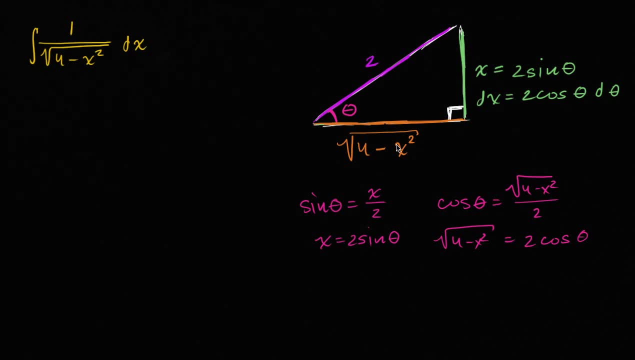 actually- let me do it in that orange color- two cosine theta. This is equal to two cosine theta And we were able to do this drawing this right triangle and using the SOHCAHTOA definition of these trig functions, and obviously we could use unit circle. 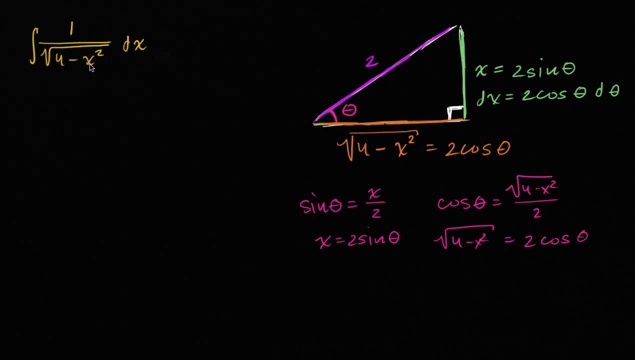 that's kind of an extension of these. but you could also do it if you say: hey, look, you know, if this is two sine theta, you could use the Pythagorean identity and you would see that this entire expression. 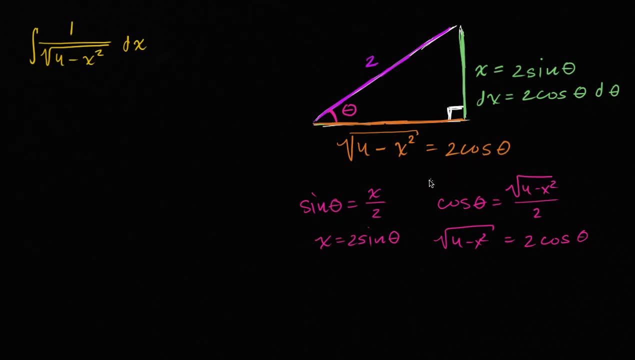 if you did it that way would simplify to two cosine theta. But now let's just run forward and let's see if we can evaluate it using this substitution. So this is going to be the indefinite integral. so dx, so one times dx, that's going to be. 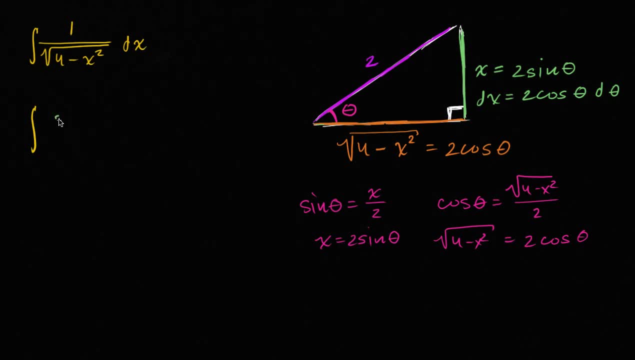 dx is two cosine theta, d theta. so let me write that That is two cosine theta. I'll write the d theta out here, and then what's the denominator Square root of four minus x squared? Well, that's two cosine theta. 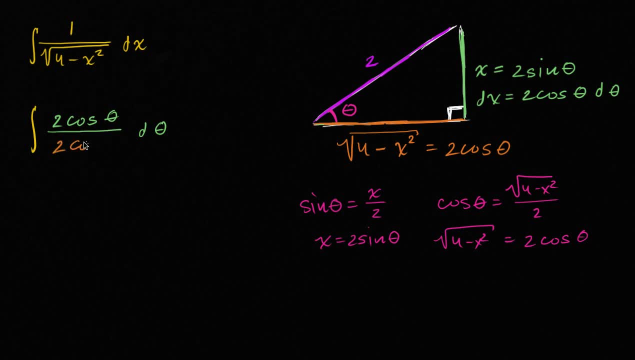 again. so that is two cosine theta. Well, this seems to work out quite nicely. If you two cosine theta over two cosine theta, that's just going to be one. This simplifies. this simplifies to d theta, which is, if you just evaluate this, 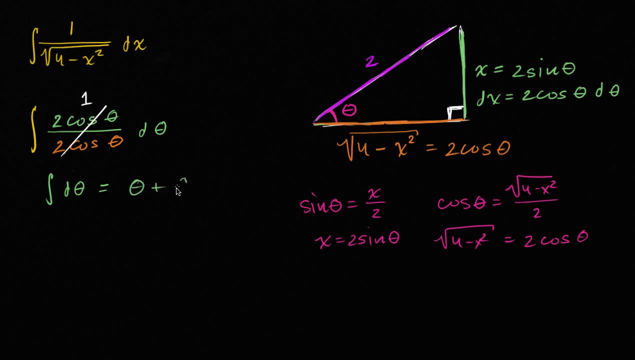 this is just going to be equal to theta plus c. Well, this is kind of nice, but we're still not done. We want this. we want our indefinite integral in terms of x. So now let's just solve for x here. 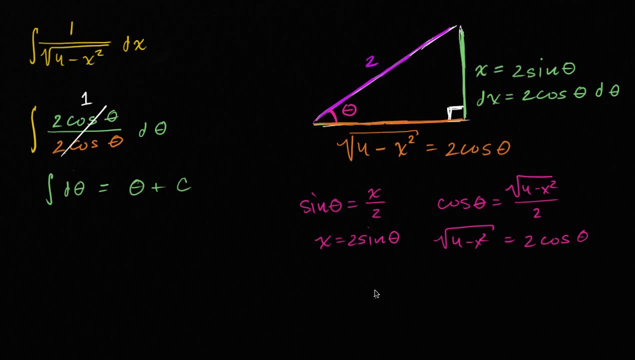 So if x is two cosine theta or, sorry, if x is two sine theta, so x is equal to two sine x is equal to two sine theta. then let's see: divide both sides by two: x over two is equal to sine theta. 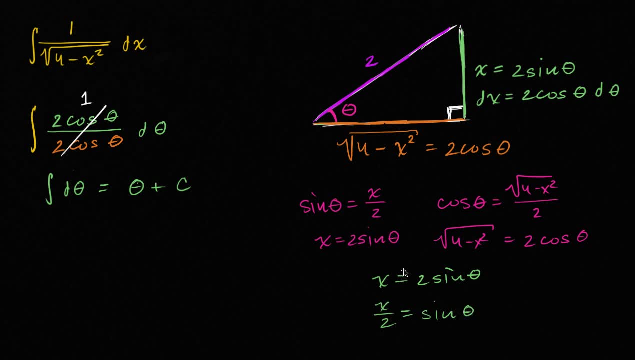 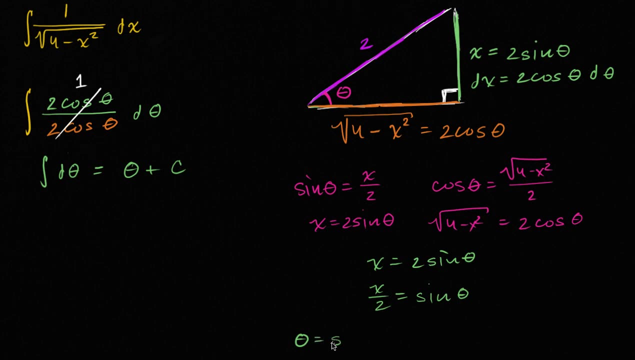 And then if you want to solve for theta, theta is the angle that if you take the sine of it you get x over two. So we could say, let's give ourselves a little bit more real estate, that theta is equal to the inverse sine. 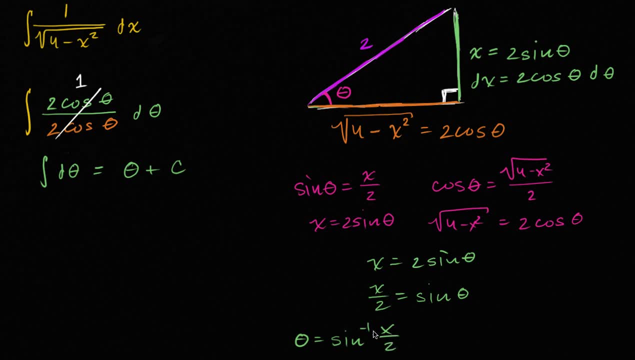 the inverse sine of this thing, x over two. We could write it that way, Or we could write that theta is equal to the arc sine, the arc sine of the arc sine of x over two. So this is going to be equal to the. 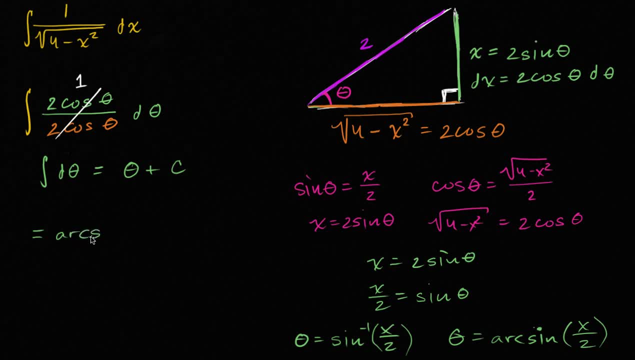 theta is arc sine of x over two. so let's just do that Arc sine of x over two plus c, And we're done. We've just evaluated that indefinite integral. Now some of you might have noticed something. I kind of brushed past it really fast. 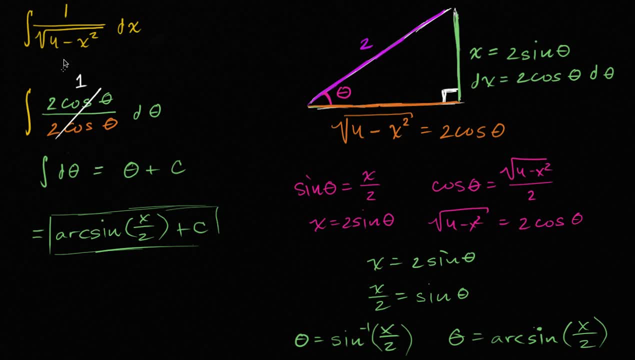 just to give you the big see: the forest for the trees. but there's some interesting details that it's, I think, worth digging into a little bit over here. So the first one is: you might see that, look, the restriction on x here is. 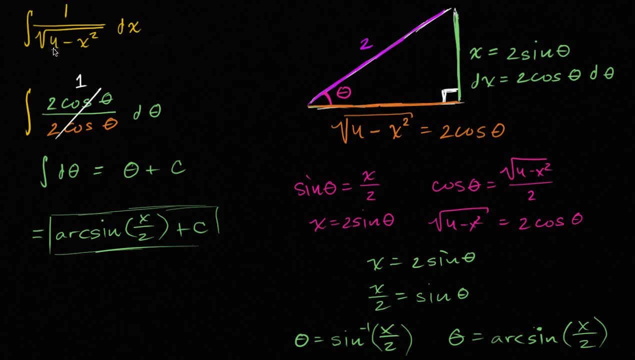 or the domain here on this expression is restricted, So let's just keep track of that to make sure that we didn't do anything strange when we did that substitution. So the domain here x has to be. x has to be greater than negative two. 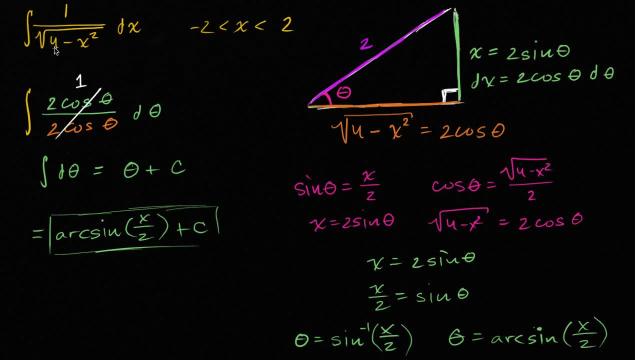 and less than two. If the absolute value of x were equal to two, then you'd have a zero in the denominator. If the absolute value of x is greater than two, then you're going to have a negative in the denominator, and that's not defined. 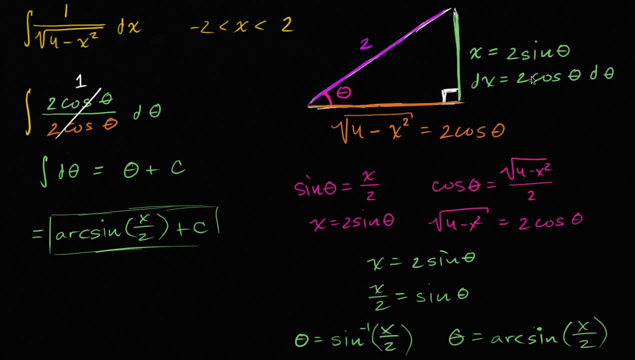 So this right over here is the domain, So let's make sure that our substitution didn't do anything weird with that. So if x has to be between negative two and two and we're saying x is two sine theta, that means two sine theta would have to be. 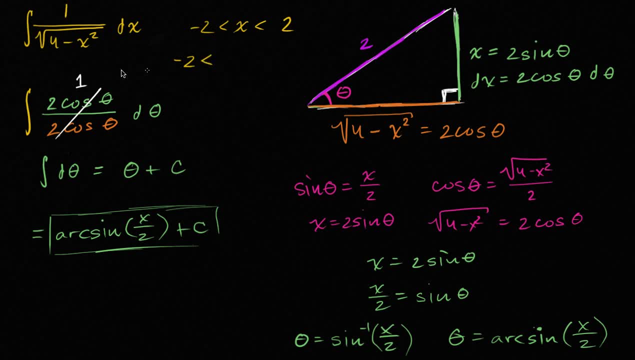 between negative two and two. So negative two would have to be less than two sine theta, two sine theta, which would have to be less than two. We could divide all the different parts of this compound inequality by two and you're gonna get negative one is less than sine theta. 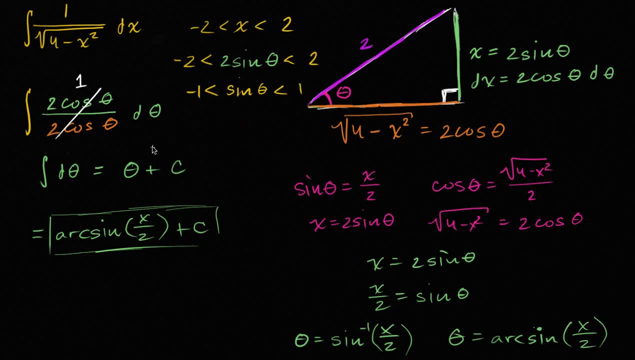 is less than sine theta which is less than one. And the way we can do that is if theta is less than pi over two. at pi over two, sine of theta would be equal to one, and if theta is greater than negative pi over two. 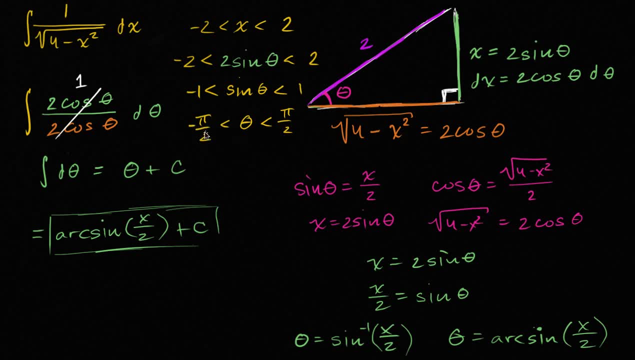 So if we restrict it in this way, if we say theta is going to be in this range right over here, then we are restricting our domain in a reasonable way And this works out well, because this typically is the range for the arc sine function, so we could feel good about that. 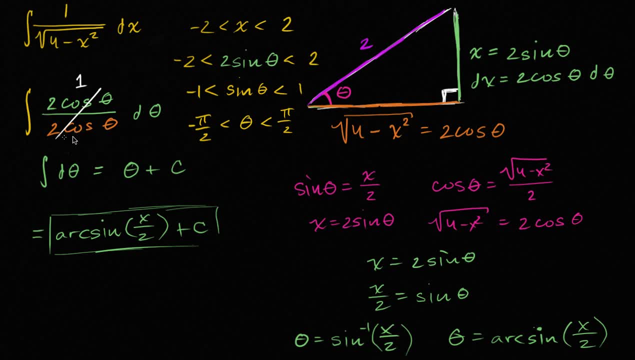 Now another question that you might have is: okay, well, look, we divided by cosine of theta here. but that's okay as long as cosine of theta does not equal zero, because you don't want a zero in a denominator. And the good thing about this restriction on theta: 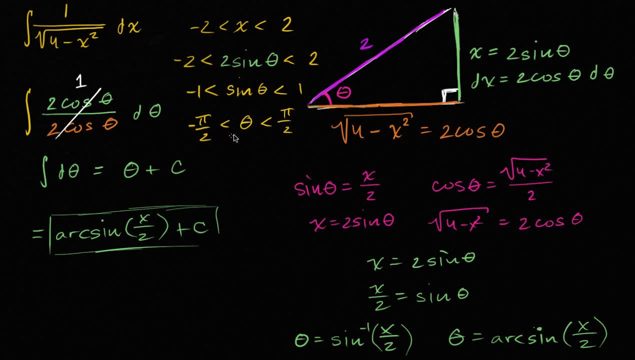 is, as long as theta is greater than negative pi over two and less than pi over two, cosine of theta is going to be, it's not going to be zero and actually it's going to be positive If negative pi over two or pi over two are allowed. 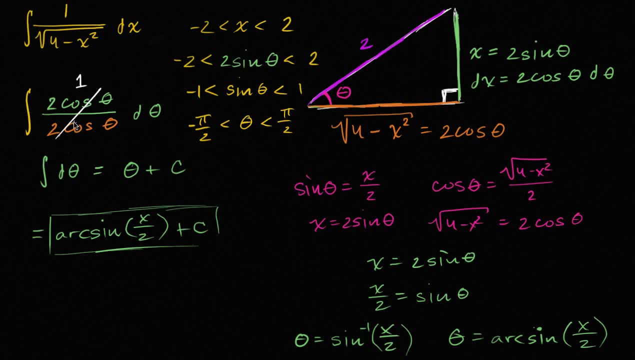 then you would get a zero down here and we would have to think about restricting things in some other ways. So it looks like everything is cool. We dug a little deeper. we said, okay, we haven't done anything strange to the domain or to the kind of unrestricted it in some strange way.